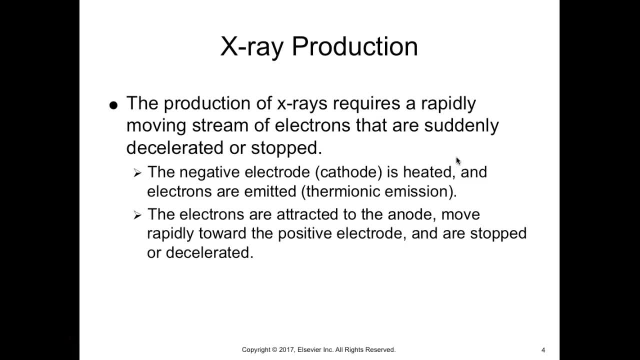 So the production of x-rays requires a rapidly moving stream of electrons to suddenly be stopped or decelerated. So the negative electrode, which is called the cathode, is heated and the electrons are boiled off. We call that thermionic emissions. 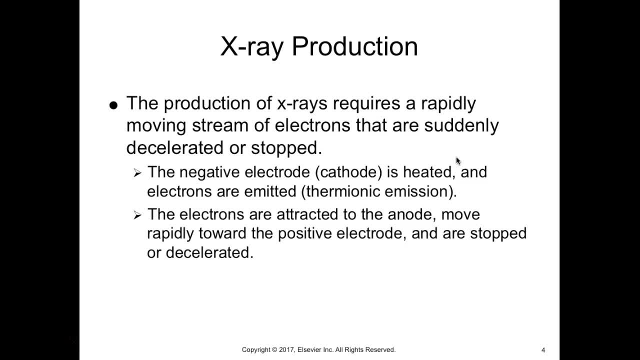 The electrons are attracted to the anode, which we'll go into in another class as to how they're attracted. So the electrons are attracted to the anode, move rapidly towards the positive electrode and are stopped or decelerated when they hit the anode. 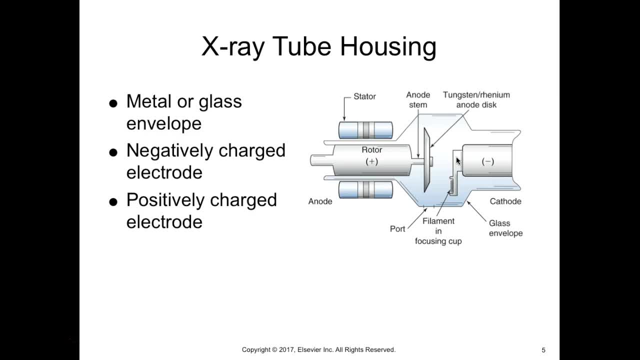 So x-rays are produced within the x-ray tube housing. So the x-ray tube housing is usually metal or glass and you can see the housing all the way around. here We have the negatively charged electrode which is here, which is our cathode end of the tube. 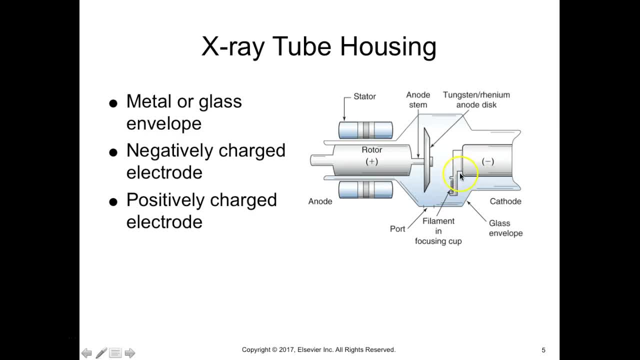 and you can see that it is negative and you can see here we have the filament. within the focusing cup, There's a port or a window within the glass or metal housing and we use that as part of our inherent filtration. There's also the positive. 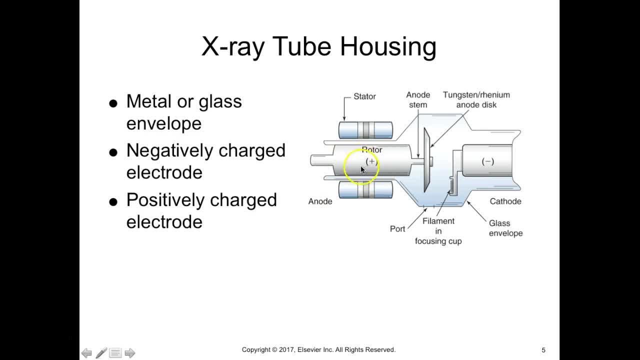 There's also the positively charged electrode, which is the rotor, and it has the stator, which is an induction motor, So it uses magnets to spin the anode. This is the anode here, This is the anode stem, and the anode is made up of tungsten and rhenium. on the disc. 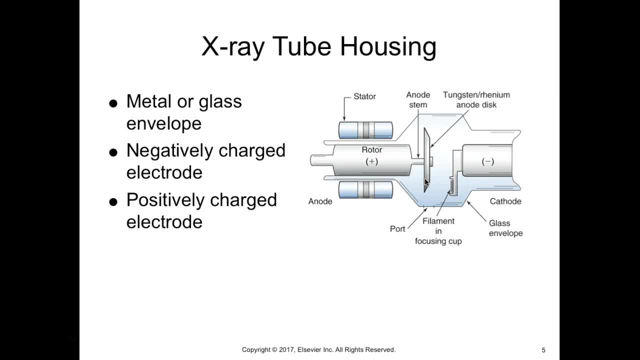 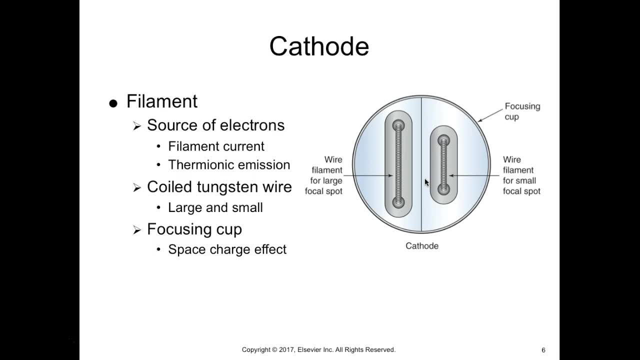 and we use the two different metals to help with the heat dissipation and the expanding and contracting of that anode. So the cathode- looking at it up close, it's the source of electrons. It has a filament current which produces your thermionic emissions and it gives us an electron cloud. 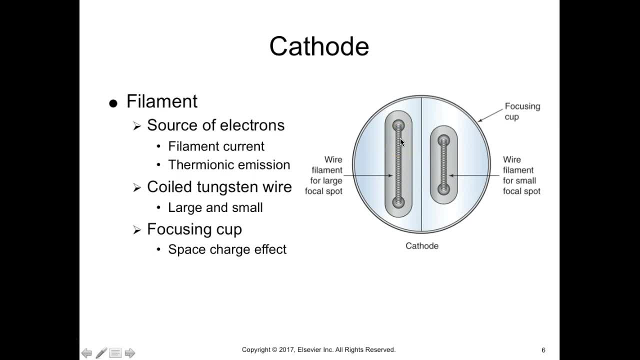 So when you're on the operating console and you see small and large focal spot, this is what we're talking about here. So we have the tungsten wire and we use tungsten because of its high melting point. So we have this small focal spot. 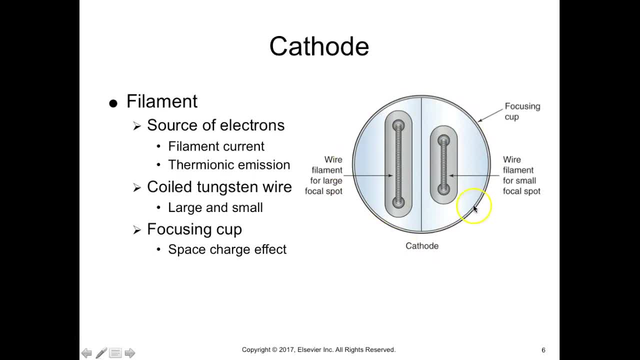 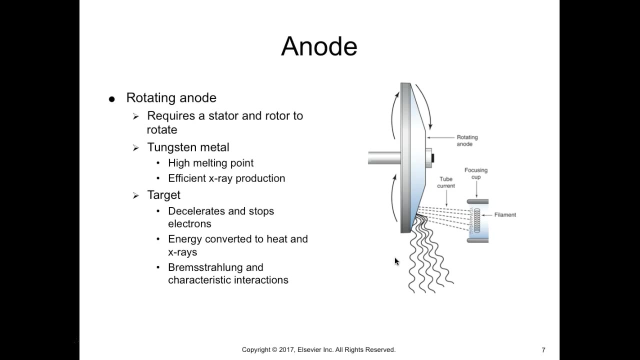 we have the large focal spot and the focusing cup all the way around and we use a focusing cup for to kind of keep the electrons within one contained area and it's for the space charge effect, The anode it rotates to help dissipate heat. so it requires a stator. 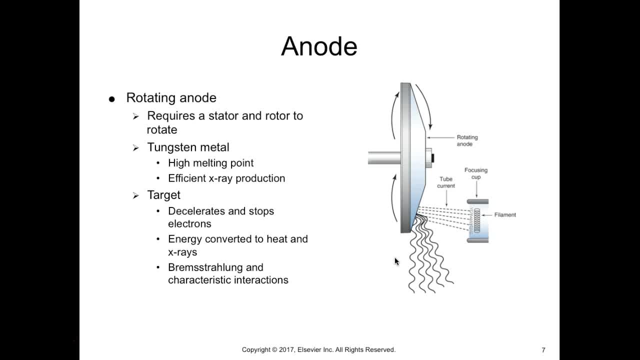 in order and a rotor for it to rotate. Like I said, the stator is on the outside of the envelope and it uses an induction motor with magnets to spin the anode. The metal that we use on the anode is tungsten and we use that because of its high melting point. 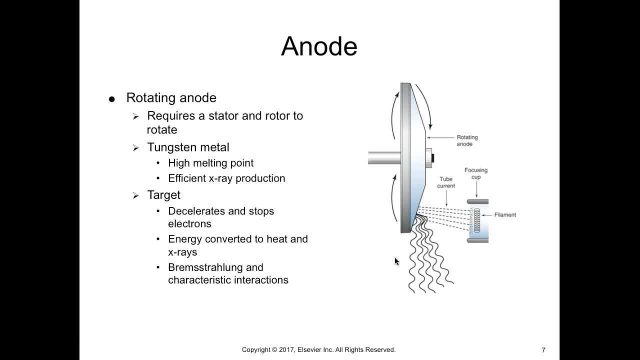 and sufficiency in x-ray production, and we'll get into that further down the road. The target is what we use to decelerate or stop the electrons from flowing. The energy is converted to heat. Remember it's 99.9% heat and less than 1% x-rays. 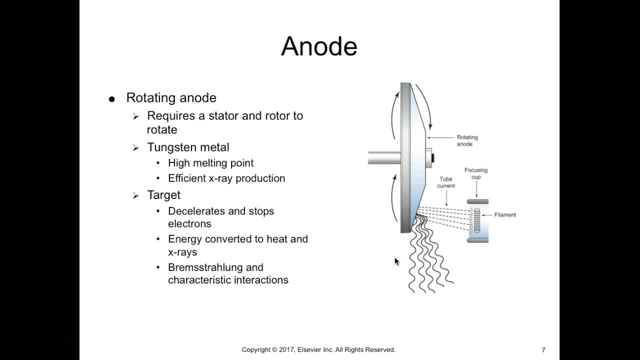 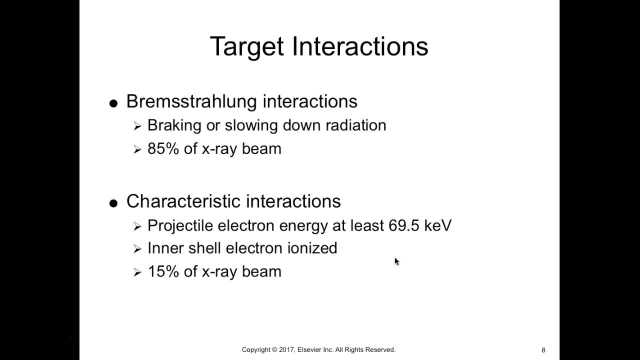 So Within the tube we have bremsstrahlung and characteristic interactions. So Bremsstrahlung interactions it's called breaking or slowing down of the radiation. So it's 85% of the beam. Characteristic interactions: a projectile: 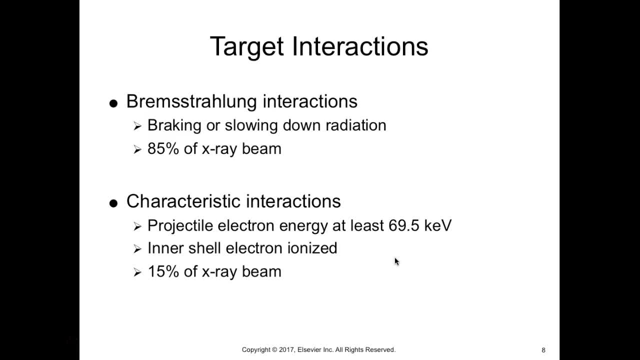 electron energy is at least 69.5 keV. When we're talking about kVp, that's kilovolts peak. When we talk about keV, we're talking about the electron energy within the tube, So keV kiloelectron volt When we have at least 69.5 keV. 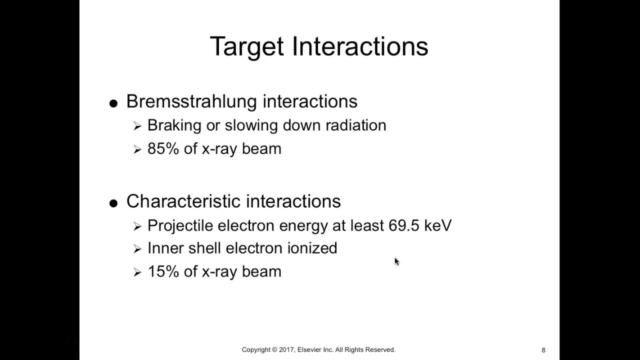 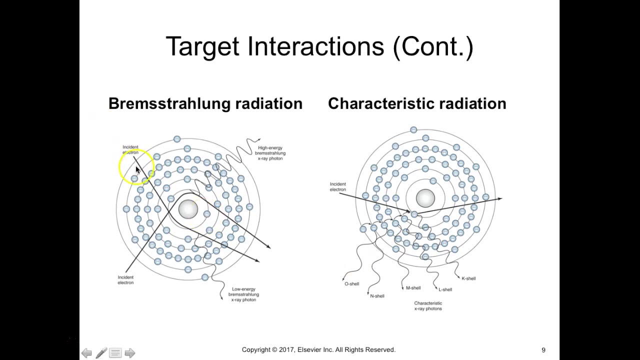 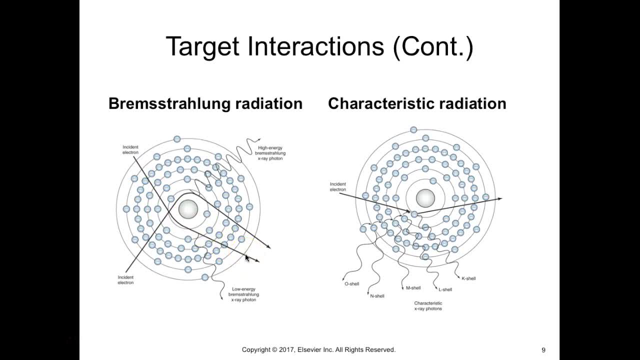 anytime there is a change in direction. we consider that a scattered photon, So it's interacted with something and is making a turn. If it has just a real slight turn, it's going to give off a lower energy: Bremsstrahlung, x-ray. 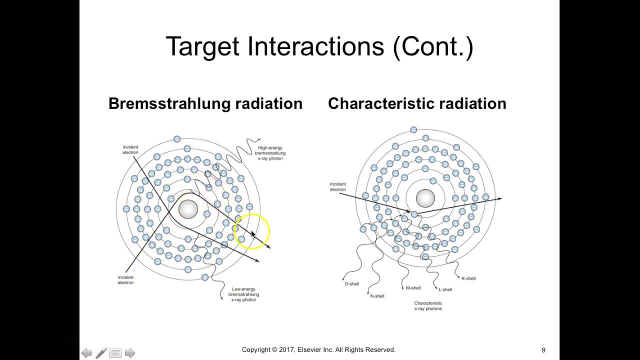 photon, Where this one you can see it's coming in and it's making a really sharp turn, so it has a higher energy Bremsstrahlung photon coming off. So with characteristic, what happens is an incident: photon comes in and interacts with an 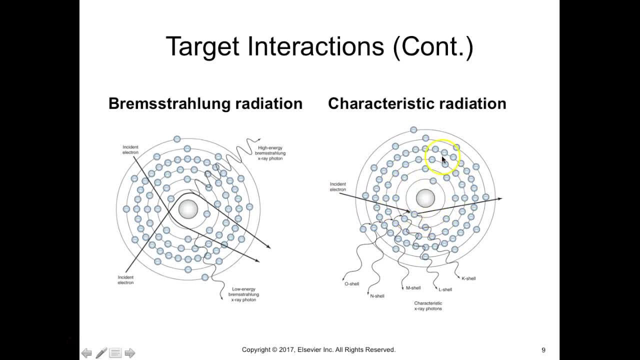 inner shell electron. So this is your K-shell, L-shell. so it keeps going K, L, M and O all the way out. So what happens is it knocks this K-shell electron out. So then the atom is very unstable. So it's going to take the L-shell and drop it down into the K and each. 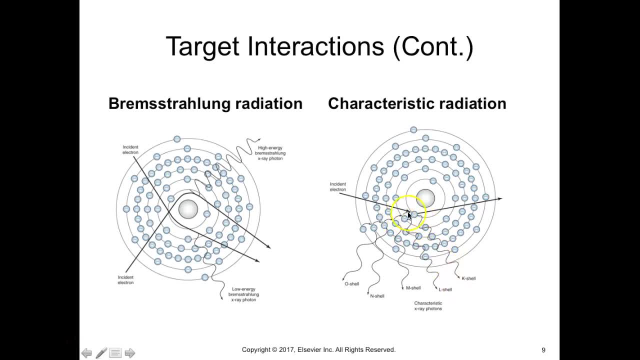 one of these photons is given off every time it drops down a level. When the electron drops down to a shell level, it drops down to a K-shell level. So it's going to drop down to a K, so it's going to drop down to a K-shell. So what happens is if the electron 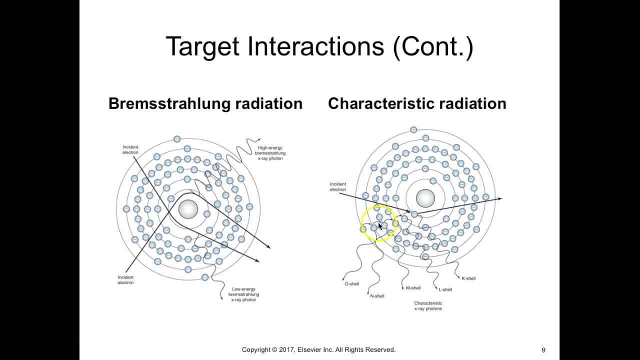 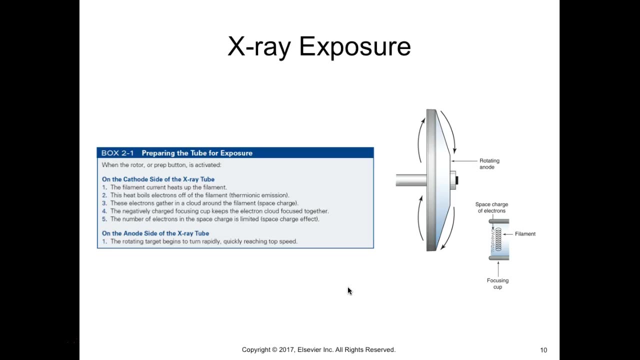 drops in a shell level that is closer to the nucleus, it gives off the photon called a characteristic X-ray photon And this whole process is called characteristic cascade. So it's cascading down, down, down, down down and giving off photons in return. So how does this work? So prepping the tube for exposure when 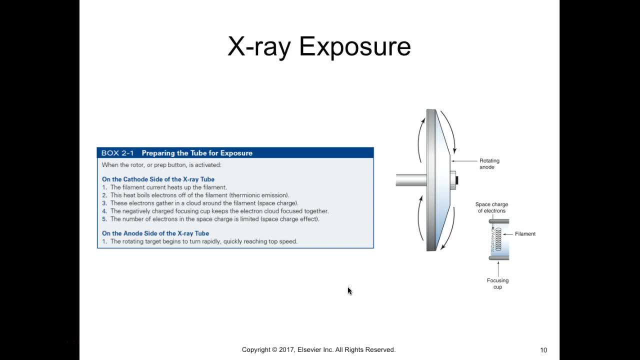 it's going to happen. so on the cathode side of the x-ray tube the filament current heats up the filament. the heat boils electrons off the filament, which is called thermionic emissions. the electrons gather in a cloud around the filament called space charge. the negatively charged focusing cups keep. 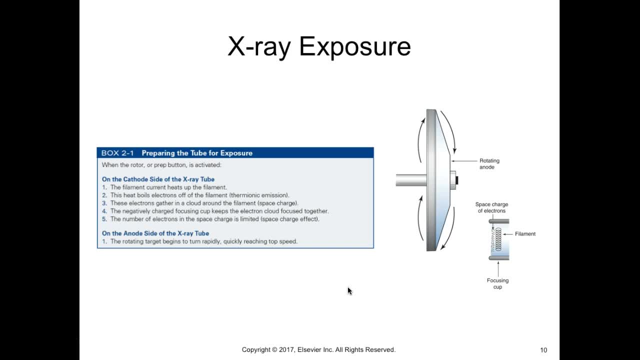 the electrons cloud together. the number of electrons in the space charge is limited. so there's it's called the space charge effect. there can only be so many electrons in that small little area. once you get to that level where you can't have any more boiling off, you've hit your space charge effect. so on the 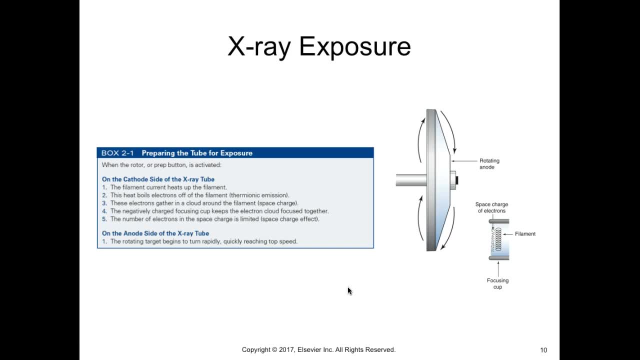 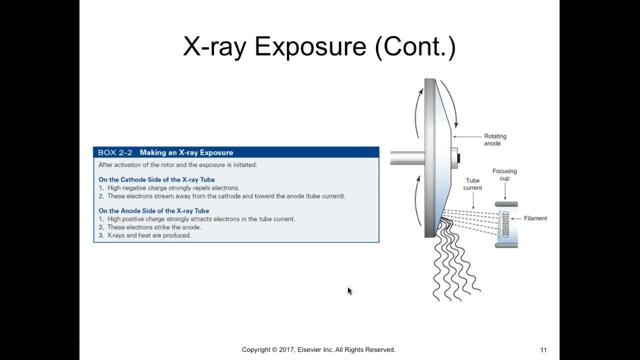 anode side of the tube. when the rotor button is prepped, the rotating anode begins to turn rapidly, quickly reaching top speed. so make an exposure. so after the activation of the rotor and the exposure is initiated. so you pushed all the way down to the top speed and the exposure is activated. so you pushed all the way down. 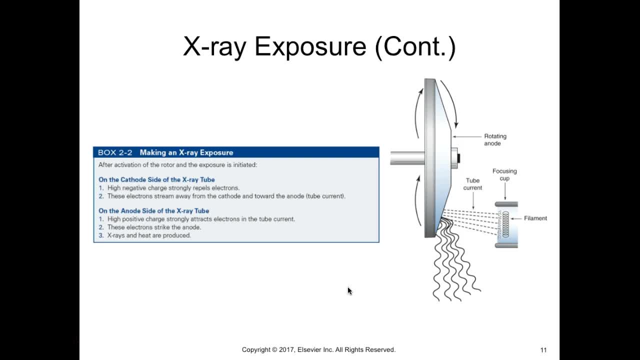 to the top speed and the exposure is activated. so you pushed all the way down on on the exposure button on the cathode side of the x-ray tube. the highly negatively charged electric- okay, so high negative charge- strongly repels electrons. so that's interesting how they wrote that. so these electron streams? 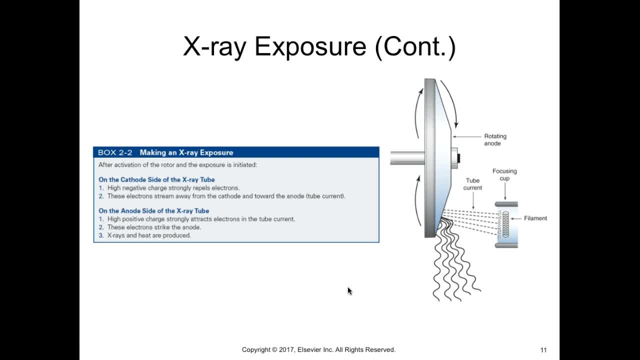 stream away from the cathode towards the anode, so that's called the tube current. so what happens is here they've got the electrons boiled off, they're within the focusing cup and so you apply, you push the button all the way down, they're pushed and pulled, so both towards the anode, to the focusing track, so on the 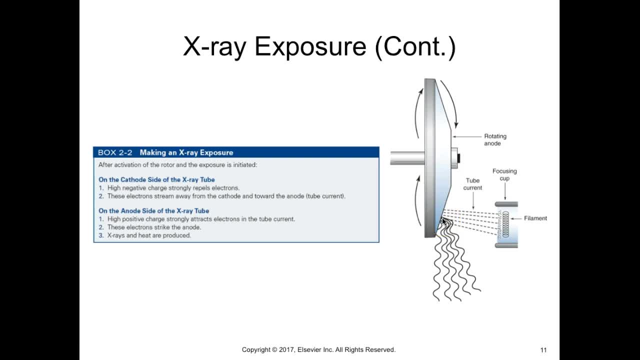 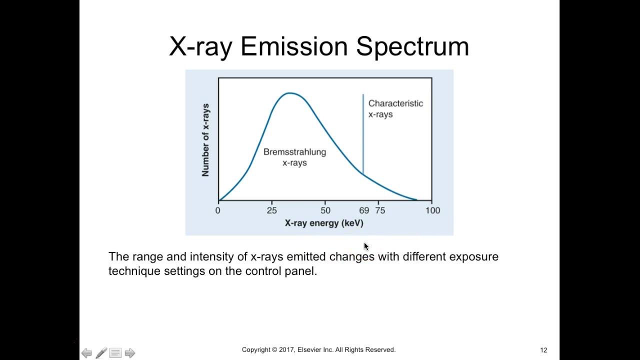 anode side. the highly positive charge strongly attracts electrons in the tube current. these electrons strike the anode, x-rays are x-rays and heat are produced. so when we're looking here at the x-ray emission spectrum, so the range and intensity of x-rays are actually very high. but the difference between the 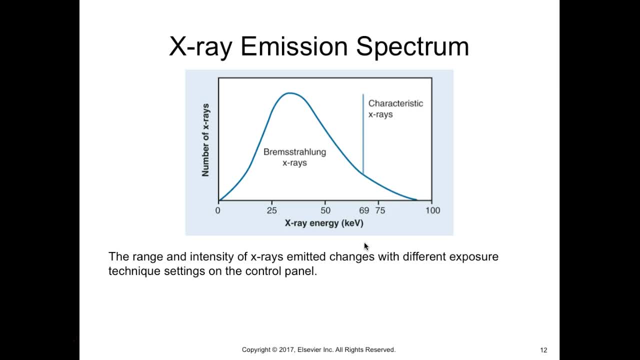 x-rays emitted change with different exposure techniques set on the control panel. so when we look in, here is your number of x-rays and here is your energy and KEV. so when we have 69.5, you're gonna see this little characteristic tick in your graph. so you have bremsstrahlung x-rays here and they stop. 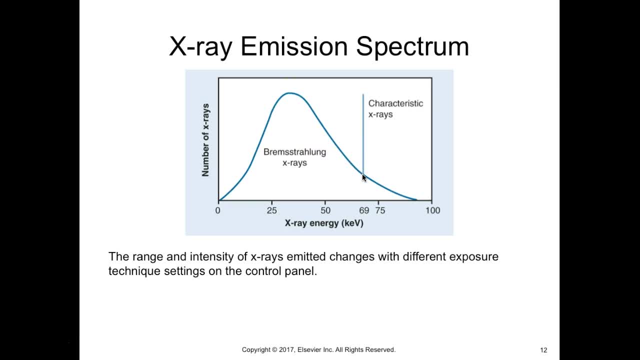 at 69.5 and higher they switch over to characteristic. characteristic cannot exist below 69.5. so that's what we're looking at here. so if you dial up, looks like 90 keV or kVp on your console. this is what your energy spectrum, your 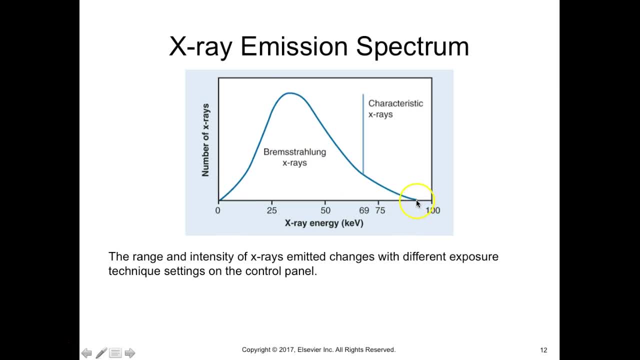 x-ray spectrum is going to look like you are only getting a couple photons. at your 90 keVp you're mainly hitting around what 34, your peak. so you have a few x-rays here and then you have a few x-rays here and then you have a few. 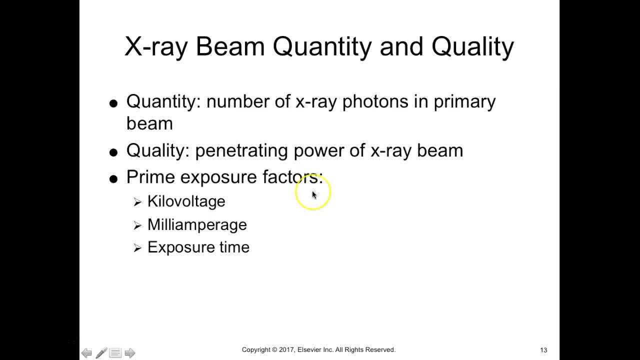 in your characteristic range, all right. so when we're talking about quantity and quality, quantity is the number of photons in the primary beam. quality is the penetrating power of the beam. your primary exposure factors are kilovolts, kilovoltage, milliampere, age and exposure time. so when we talk about kilovoltage, 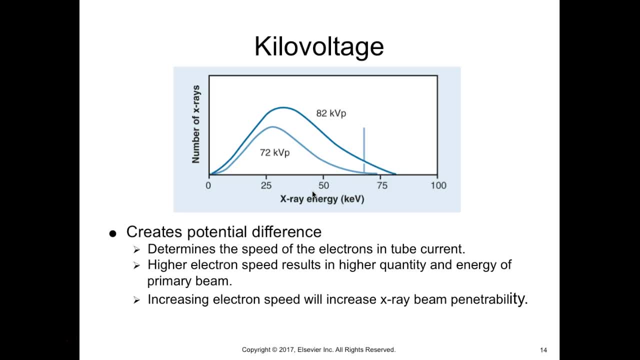 it creates a potential difference, so it determines the speed of the electrons in the tube current. so higher the electron speed results in higher quantity of energy of the primary beam. increasing the electron speed will increase the beam penetrability. so when you set your kVp to 72 you can see your x-ray. 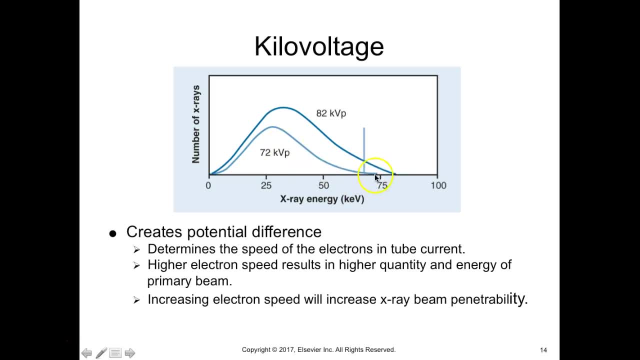 spectrum here. if you set or yep 72, so if you set it at 82, you can see you have a higher power, a higher energy x-ray beam. so what's this tick yep characteristic milliampere age. so the unit to measure tube current or the 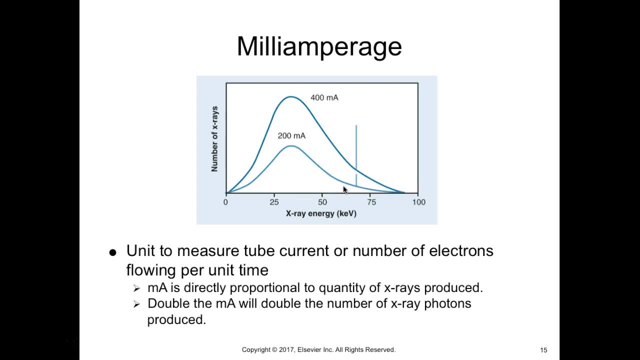 number of electrons flowing per unit of time. so ma is directly proportional to the quantity of x-rays produce. so you double the ma, you double the number of photons produce. so here you can see, we've got our tick there: 69.5. we have 200 ma, we have 400 ma, directly proportional. 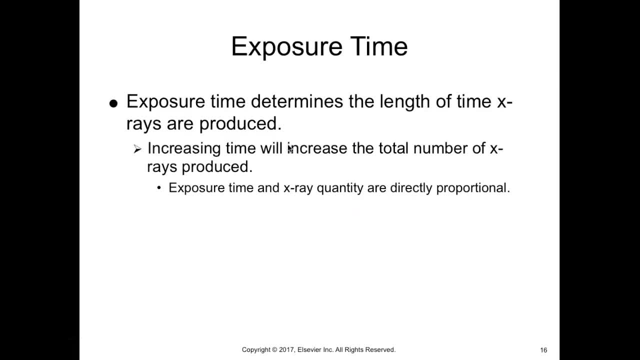 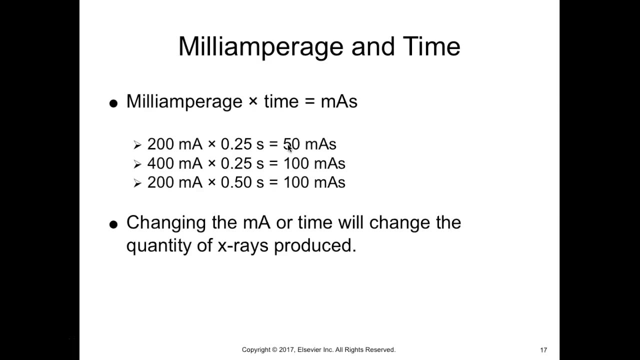 if you double the, the number, you double the amount that you're going to be producing. so exposure time: exposure time determines the length of the time the x-rays are produced. increase in time, we'll increase the total number of x-rays produced. exposure time and x-ray quantity are directly proportional. so 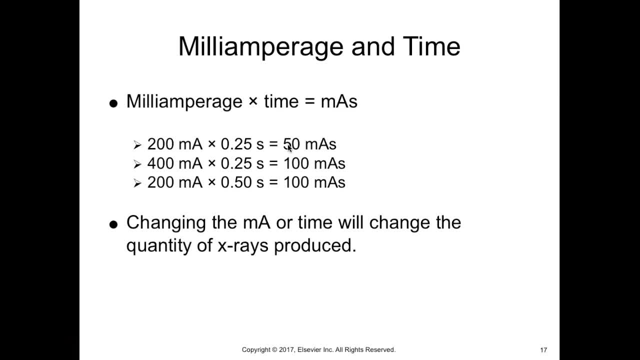 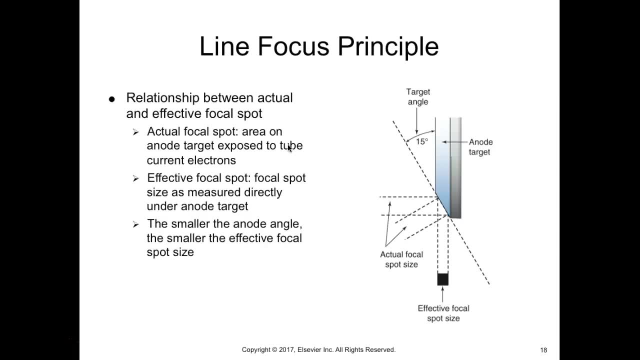 here's some examples. so, milliampere, each time is your ma ass. so changing the ma or the time will change the quantity of the x-rays produced. line focused on time: you can see at interlink started on the line focus principle. okay, so this is this is a concept, this is something that 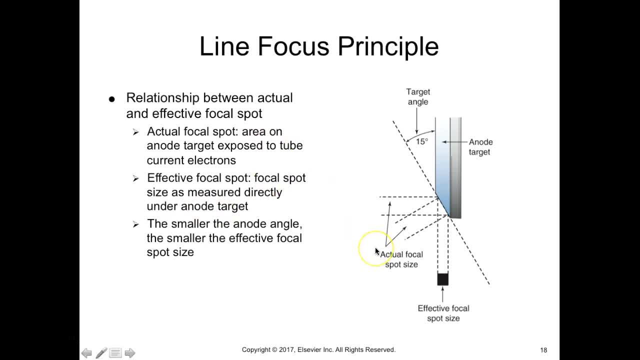 we will go further into later on, but I want you to be introduced to it. so line focus principle is a relationship between the actual and effective focal spot. so the actual focus spot is the area on the anode target exposed to the current of electrons. so these- this right here- is electrons coming in to hit the 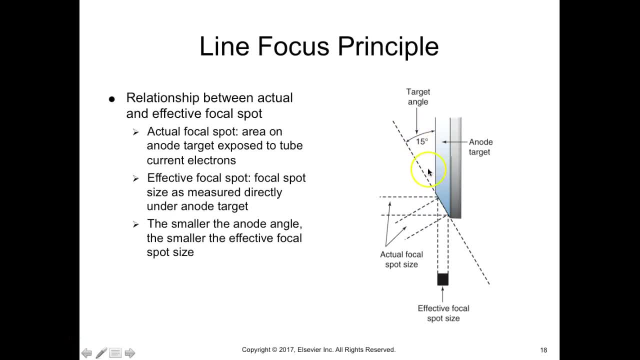 target. so this is your target. right here we have a 15 degree angle, so electrons come in. this is your actual focal spot size. now, since it's at an angle, the effective focal spot size coming off is going to be smaller. so the effective focal spot size is measured directly under the anode target. so it's right. 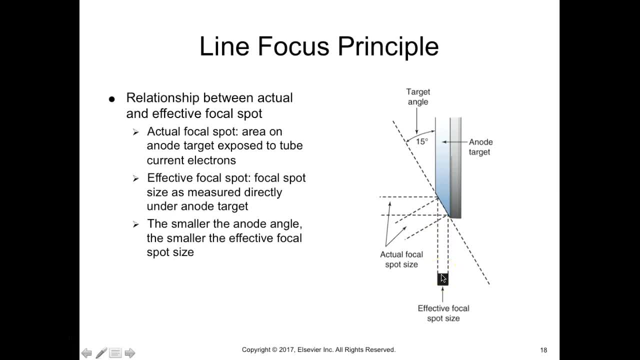 underneath it. the smaller the anode angle, the smaller the effective focal spot. so as the anode target is measured, the smaller the effective focal spot, so as the this gets smaller, as it goes from 15, let's say, to 5% or 5 degrees. this will be. 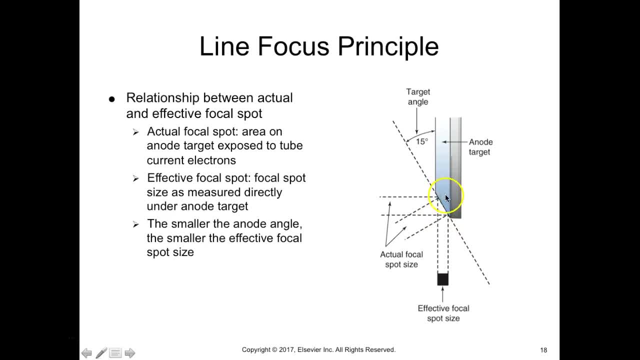 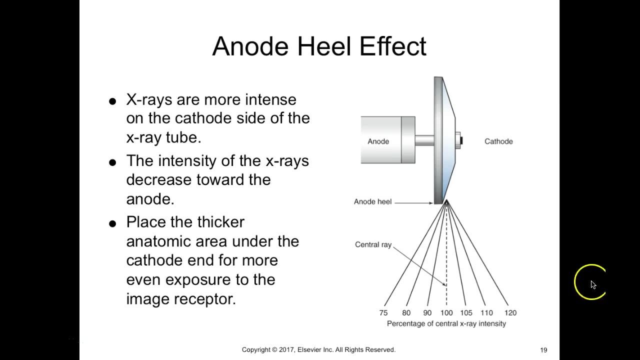 narrower. this will be smaller if it the angle goes to 30, so these electrons have more area to hit, so it's going to be bigger coming off. all right, the anode Hill effect. I think we've talked about this before. so you have your anode, you. 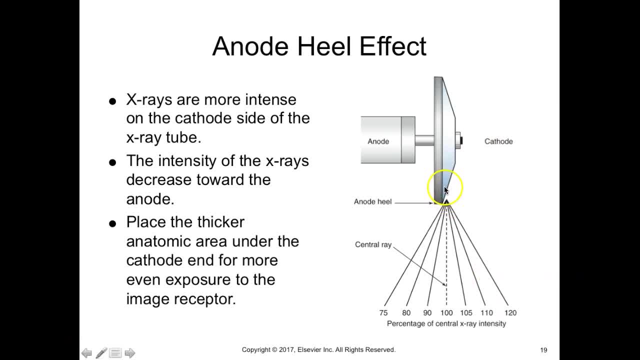 have your cathode. your electrons are hitting your focal track and they're coming off. now they come off at an angle and they're coming off with a varying degree of intensity. so x-rays are more intense on the cathode side of the x-ray tube. so this is the cathode side over here, so you can see I have a hundred. 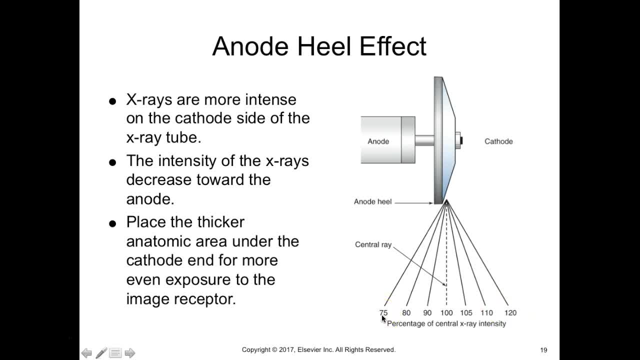 twenty for the intensity, compared to 75 over here. so the intensities, the intensity of the x-rays, decreased towards the anode. so what you want to do is you want to place the thicker portion of the body part toward the cathode side. so one way to remember is fat cat, so cat for. 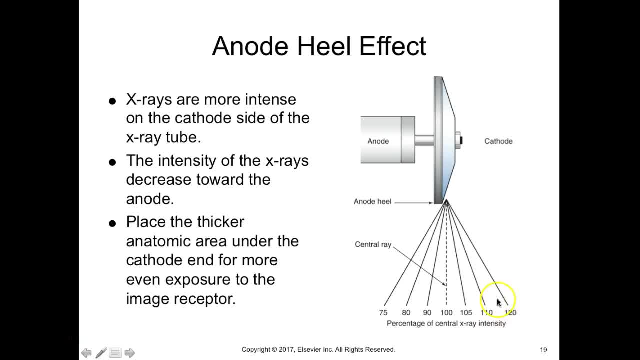 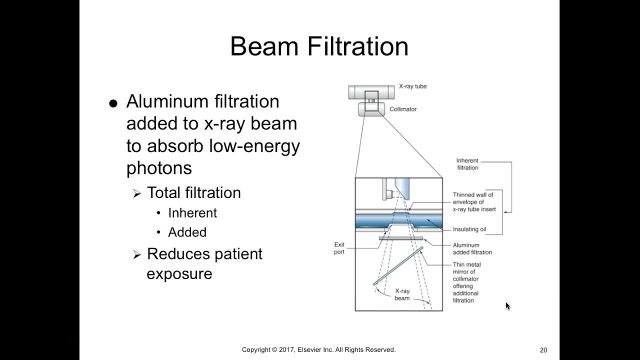 cathode and fat. so think of the thicker side towards the cathode side filtration. so we use aluminum, we add it to the x-ray beam to absorb low energy photons. so, looking here, we have the total filtration inherent plus the added. and why we do this is to reduce the patient's exposure. 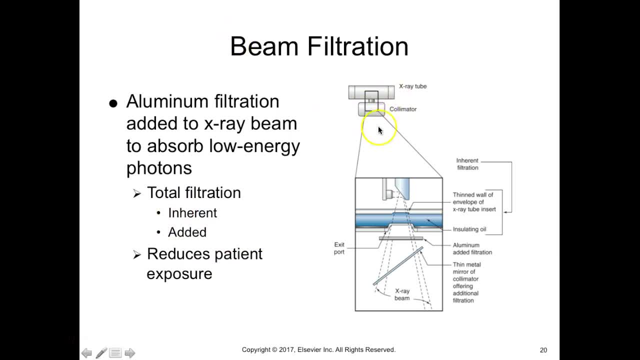 so it'll reduce skin dose. so here within the x-ray tube, you have the collimator. we're gonna blow it up and you can see, here we have, where are we. we have the oil that's gonna absorb some of the lower energy. we have an aluminum filter. 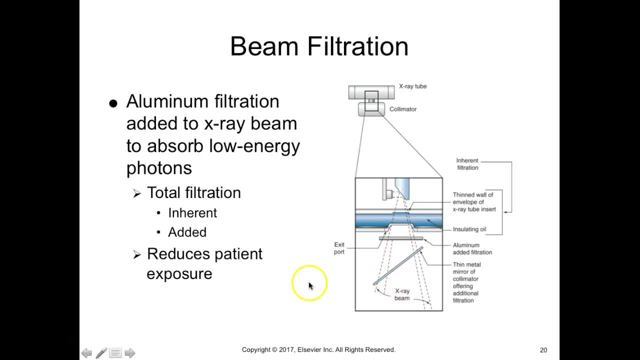 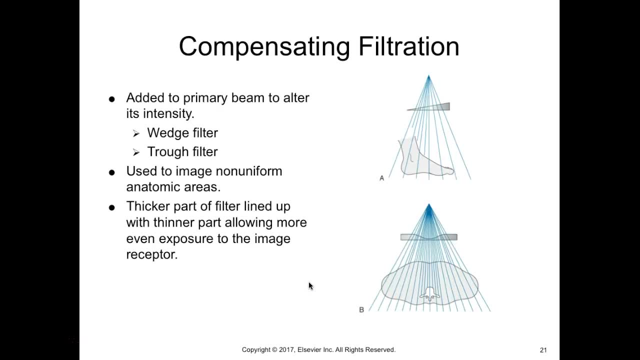 and we have a mirror all together. the filtration is used to reduce patient dose, so we can use additional filters as needed for patients. so I just want you know the basic concepts of it. so adding two primary beam to alter its intensity, so wedge filter, and there's a trough filter. so for a wedge filter, as you can. 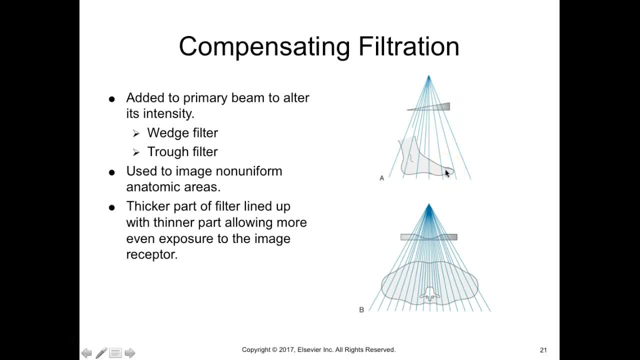 see, you put the thickest part over the thinnest subject part, that's the subject positioning. so here the thinner parts going to the thicker. so here, with the trough filter, the mediastinum is pretty dense, so the lungs are not, so we'd use a. 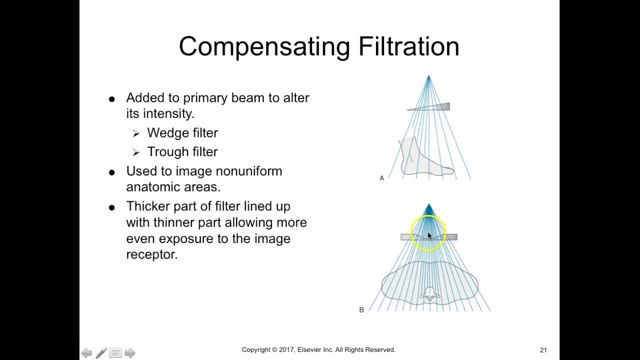 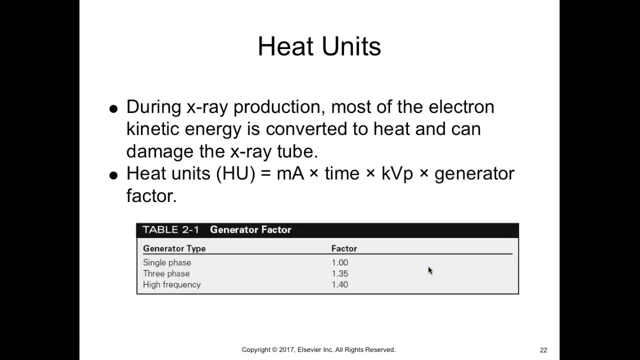 trough filter. this is called trough filter so that we could see the lungs and the mediastinum properly exposed. all right, heat units. why do we have to worry about heat? so during x-ray production, most of the electron kinetic energy is converted to heat and can damage the x-ray tube. so how do we figure out what? 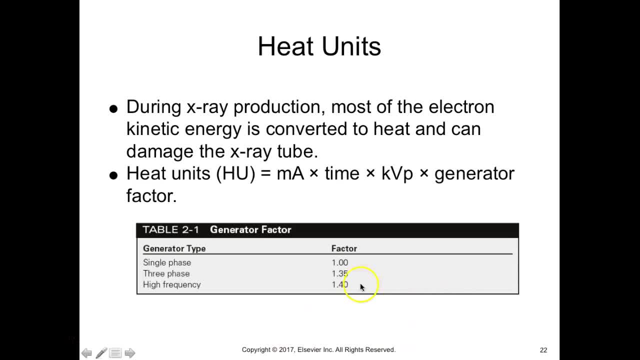 the heat units are. most of us are using high frequency generators. I can't imagine anyone using less than a high frequency generator. I suppose they could be out there still, but your equation is going to be 1.40. so what you're going to do to calculate your heat units? you're going 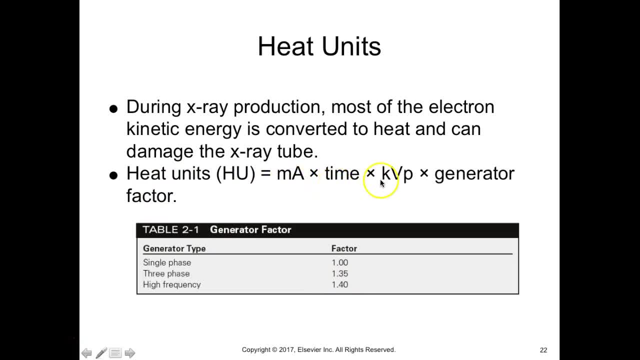 to take your ma times, your time or your mas, multiply it by your kVp and multiply it by your generator factor, which is 1.40, and that'll give you your heat units. and then there's graphs that you can check to make sure that you're not going. 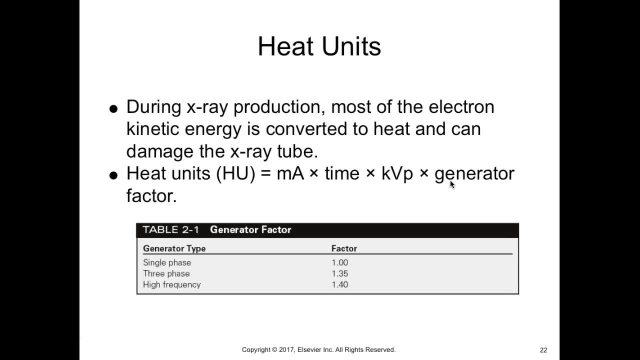 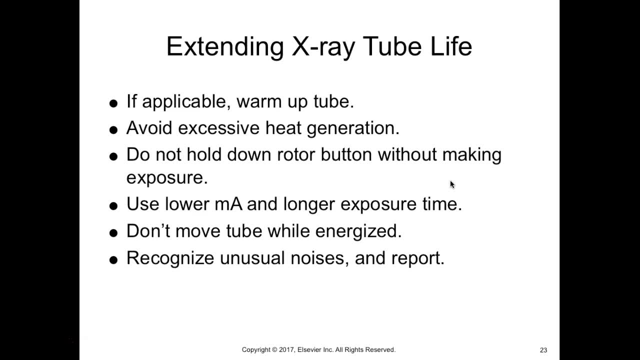 to damage your tubes when you're making exposures. so to extend the x-ray tube life you'll want to warm up the tube if it's been sitting and it's a cold tube and you get a patient and you're doing a lot of x-rays- really high-energy x-rays- you 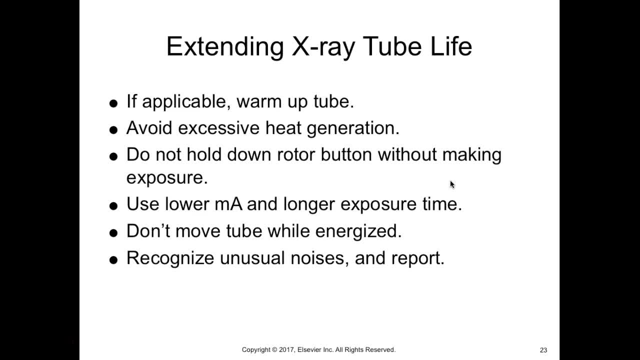 could actually crack your tube. you can crack your anode. there's all things, all bad things, that can happen, so you'll want to warm up your tube if it's been sitting for a long period of time. you want to avoid excessive heat generations and don't hold down the rotor button.